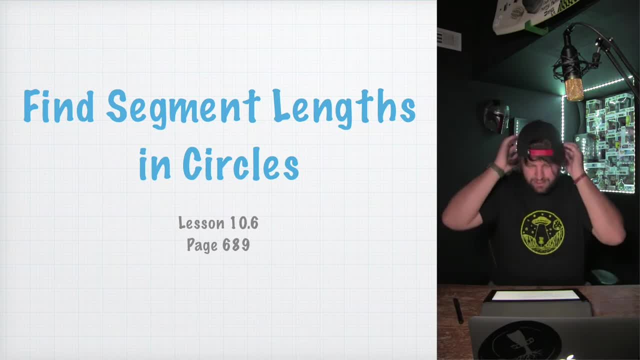 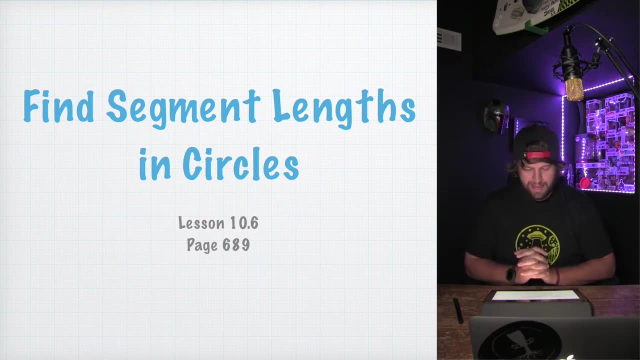 have a great day In Jesus' name. I pray Amen. All right, you guys. So today we're going to be learning how to find segment lengths in circles. This is lesson 10.6, page 689.. So here we go. 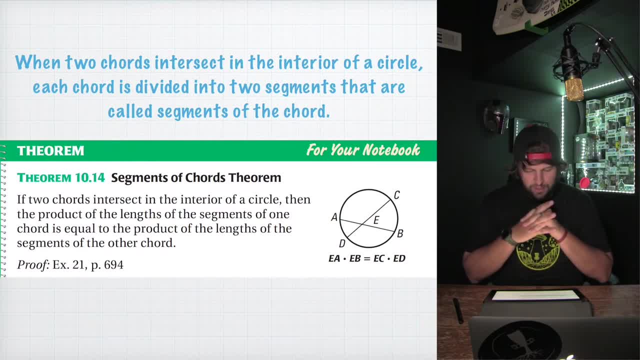 When two cords intersect in the interior of a circle, each cord is divided into two segments that are called segments of the cord. So theorem 10.14 says segments of cords theorem. If two cords intersect in the interior of a circle, then the product of their lengths of the segments of 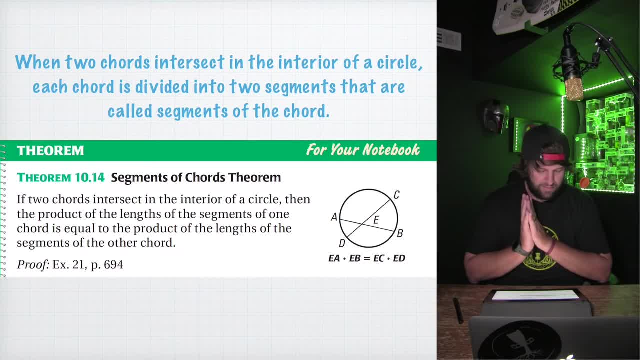 one cord is equal to the product of the lengths of the segments of the other cord. So here you go. You know that AE times EB should equal CE times ED. That's what theorem 10.14 says. So let's go ahead and try that. They want us to find RT and SU. Well, to do that, we're going to have to find. 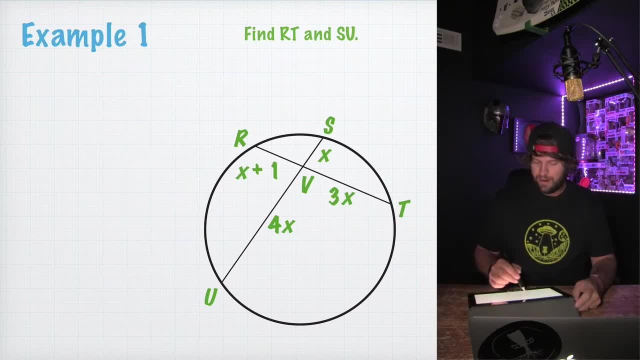 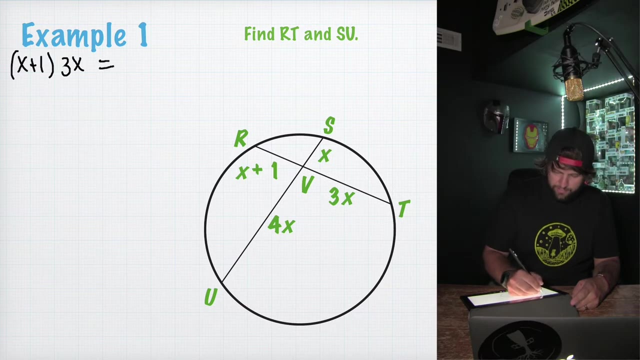 that We're going to have to solve for X, And we know that RV times VT should equal SV times VU. So X plus 1 times 3X should equal 4X times X. Okay, So if we were to FOIL this out, 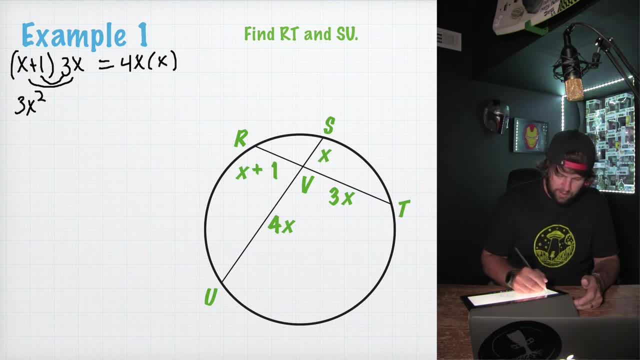 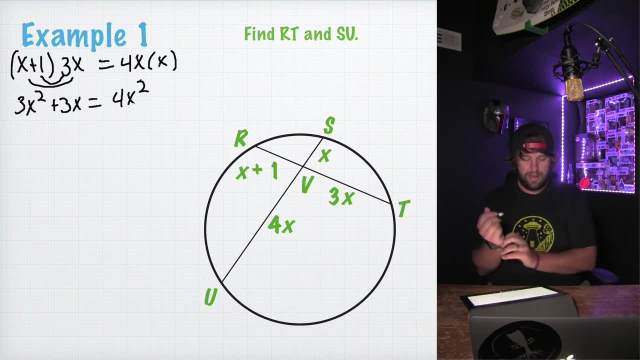 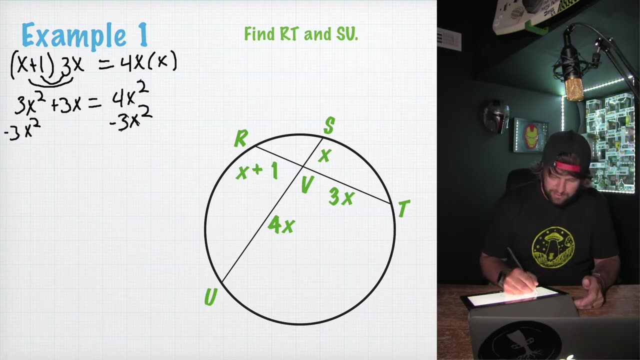 3X times X is going to be 3X squared plus 3X equals 4X squared. Let's go ahead and subtract 3X from each side. 3X squared from each side. Sorry, That's going to cancel out. We're going. 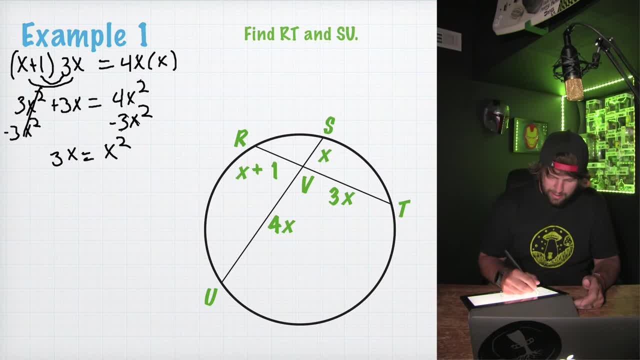 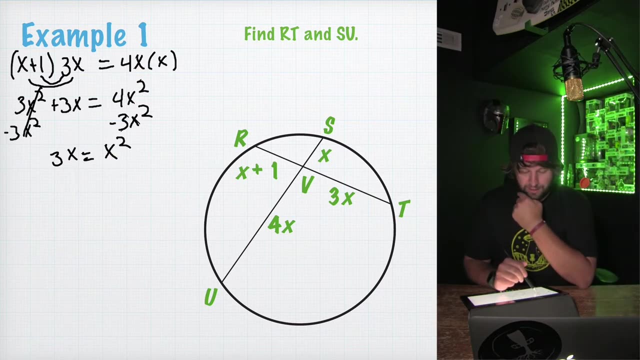 to be left with 3X equals X squared. Okay, Now, this kind of looks a little confusing, possibly, but to get X squared, we know we just simply multiply X by X, right? So if we were to divide each side by X so you get rid of the X on the 3,, we'd be left with just 3 equals X, because X times. 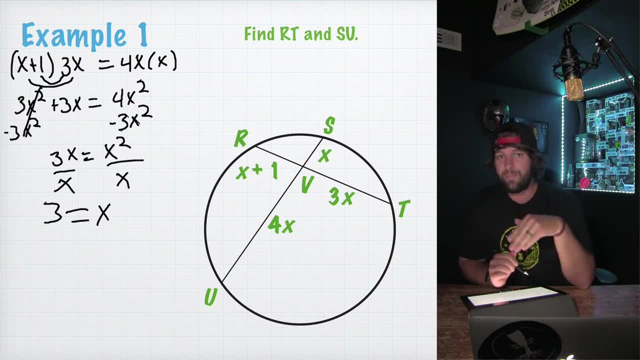 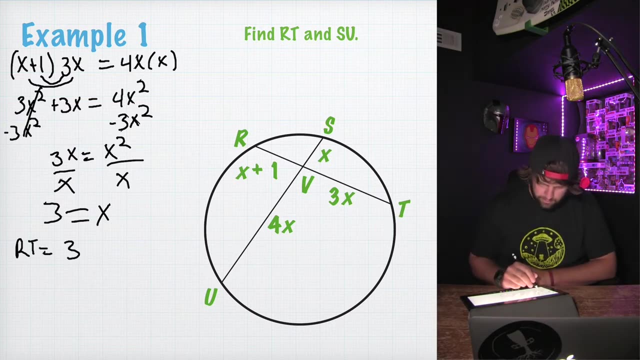 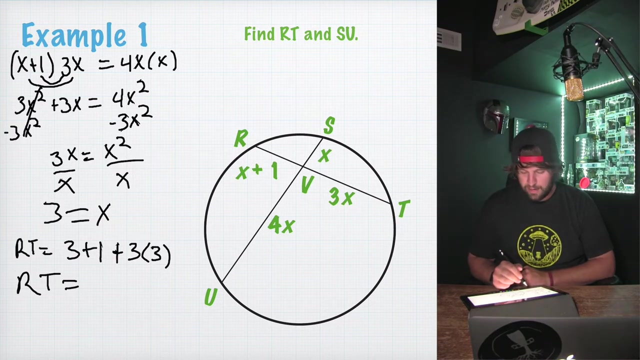 X equals X squared, So it makes sense: X squared divided by X just equals X, So X equals 3.. Now we're not done. They want us to solve for RT and SU. So RT is going to equal 3 plus 1 plus 3 times 3.. So RT is going to equal: 3 plus 1 is 4.. 3 times 3 is 9.. 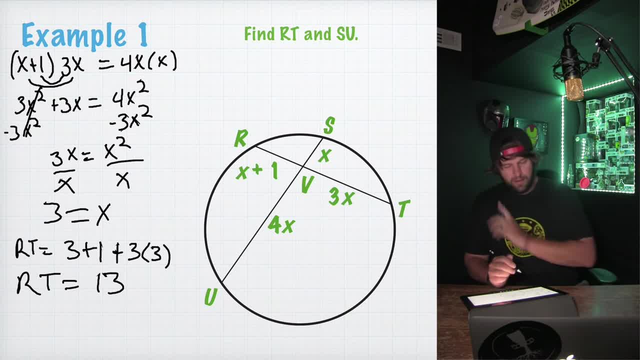 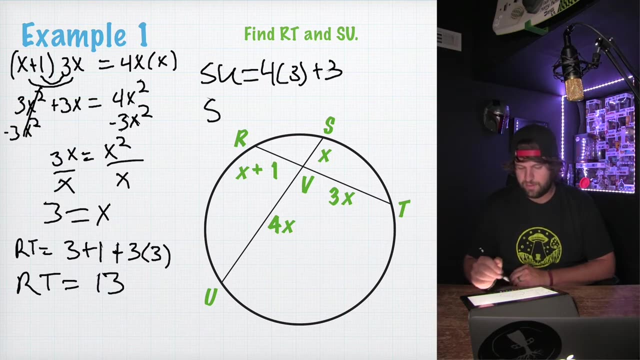 So 13.. Okay, And then let's go ahead and do SU up here. SU should equal 4 times 3 plus 3. Okay, So 12 plus 3 is 15.. SU equals 15.. Okay, That's example one and done. 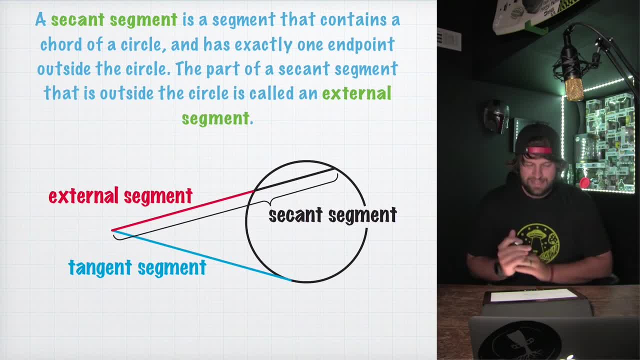 and in the book. So let's keep going. A secant segment is a segment that contains a chord of a circle and has exactly one end point outside the circle. The parts of a secant segment that is outside the circle are the parts of a secant segment that is outside the circle. 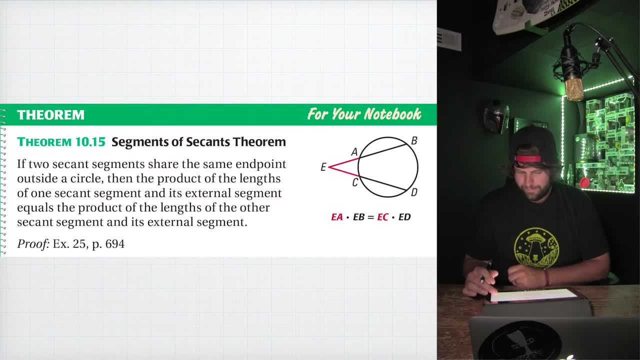 It's called the external segment. Okay, So theorem 10.15 says segments of secant's theorem. If two secant segments share the same end point, so like these share E, then the products of the lengths of one secant segment and its external segment equals the product of the lengths of the 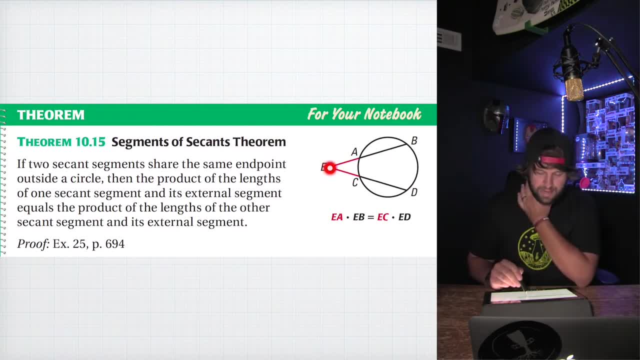 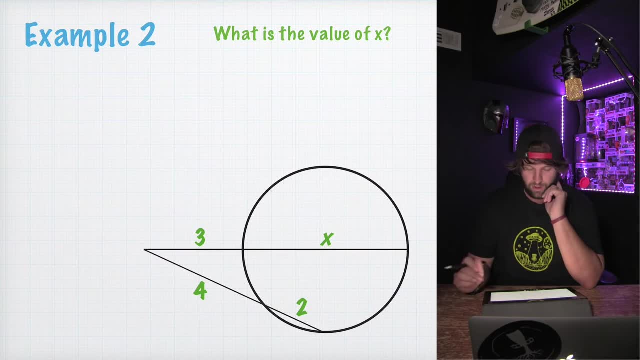 other secant segment and its external segment. So EA times the full length EB should equal EC times the full length of EC. So the product of the length of the external segment equals the product of the external segment. So here we go. What is the value of X? We have 3 times, and now it's not just X. 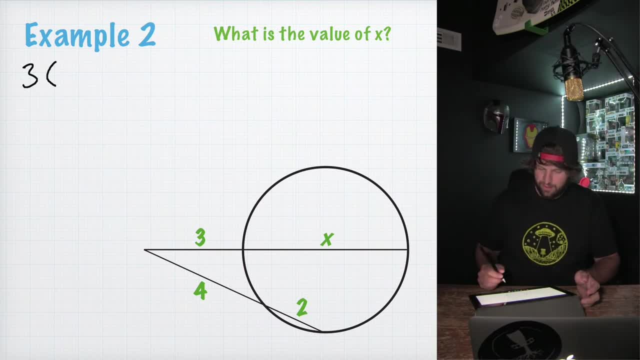 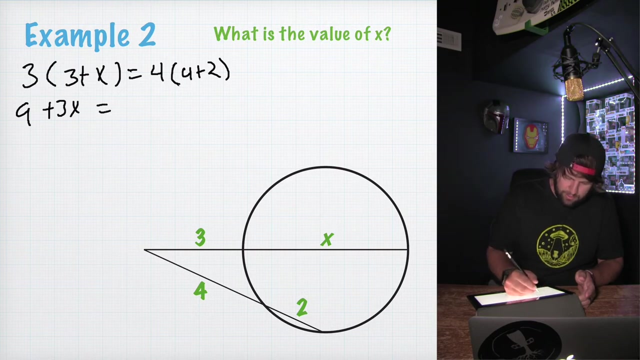 it's 3 plus X because it's multiplying by the full length. So 3 times 3 plus X equals 4 times. I'm just going to write it: 4 plus 2, which would be 6.. So we got to FOIL this, or distribute it, whatever you want to call it. 3 times 3 is 9 plus 3X equals. 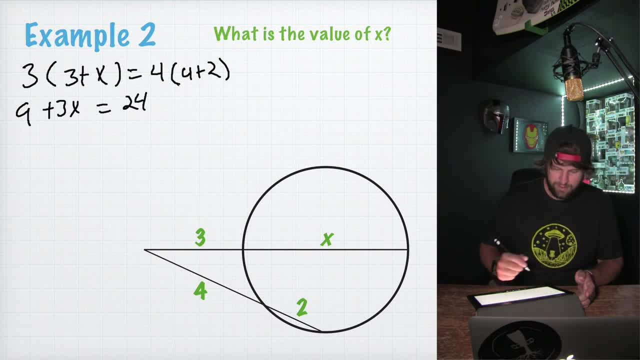 6 times 4 is 24.. Sometimes people want to do 4 times 4 and 4 times 2, but just remember, PIMDAS says that we can add this first. should add this first: 4 plus 2 is 6 times 4, then 24.. 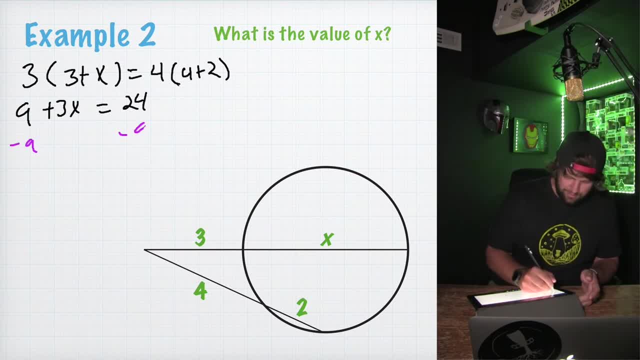 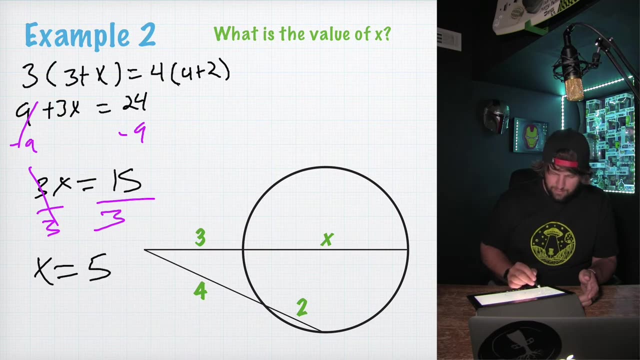 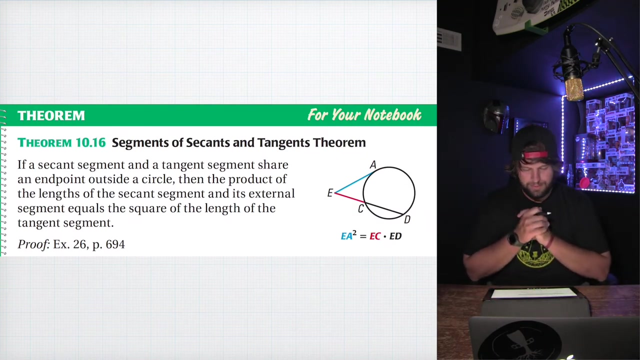 You do that and see how easy it is, Subtract 9 from each side. Now that 9 is cancelled, we're left with 3X equals 15.. Divide by 3. And X equals 5.. Example 2, let's keep going- 10.16.. Segments of secants and tangents: theorem. If a secant segment is less than 4 versus 2 X, it means its signal is less than 2 as long as it's less than 2.. Then if G is less than 2,, then it's lower than 5.. At the moment of the solution. 1 minus G is less than 2.. Let's go ahead and do 2.. We can defeat the sixteenth and dimensionseny for which we see about all quadrat cited as different approaches for Y's. The second example is a n-andAI where G is greater than 1 by 4 of X. 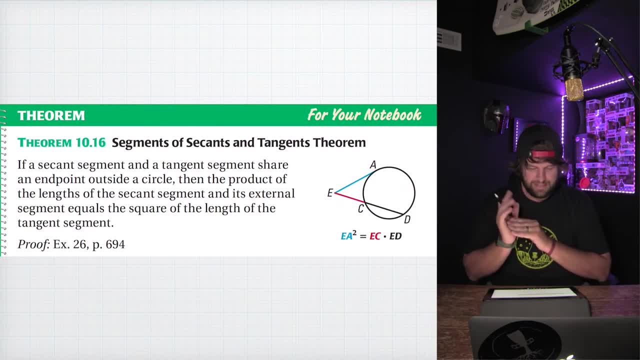 and tangents theorem. If a secant segment and a tangent segment share an endpoint outside a circle, then the product of the lengths of the secant segment and its external segment equals the square of the length of the tangent segment. So the tangent right here, EA, if you square that. 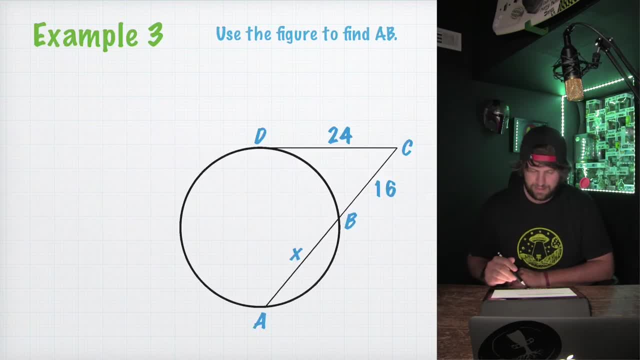 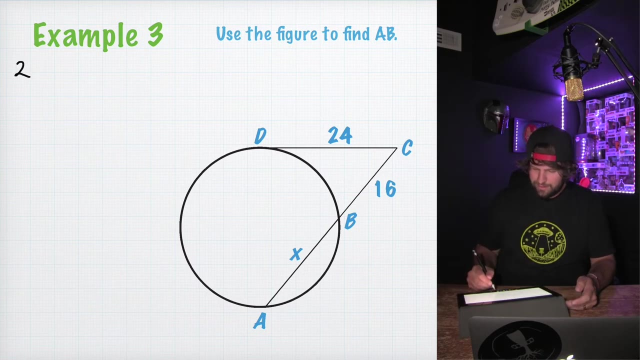 should equal EC times its full length, ED. So let's give that a shot. We know that 24 squared should equal 16 times the full length, which is 16 plus X, So let's go ahead and write this down: 24 squared should equal 16 times 16 plus X. Okay, so 24 squared is going to be: 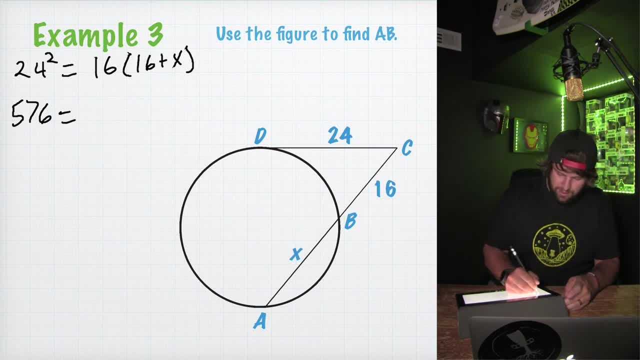 16 times 16 plus X. So 24 squared is going to be 16 times 16 plus X. So 24 squared is going to be 576.. 576 should equal 16 times 16, 256, plus 16X. Okay, subtract 256 from each side. 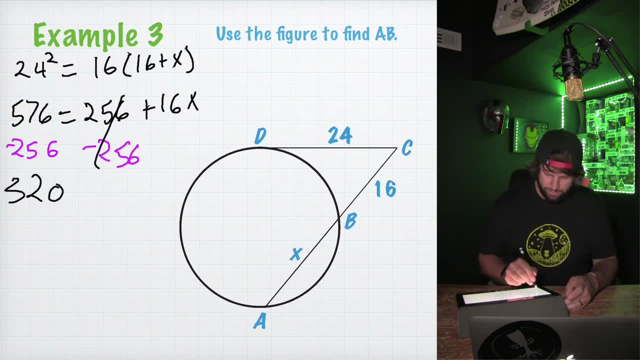 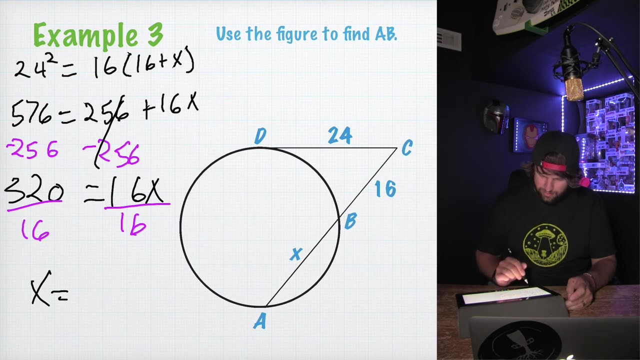 We're left with 320, and that canceled out. so it equals 16X Divide by 16, and X equals 20. And 20 equals AB. Okay, So that's how we do that one. Let's keep going. 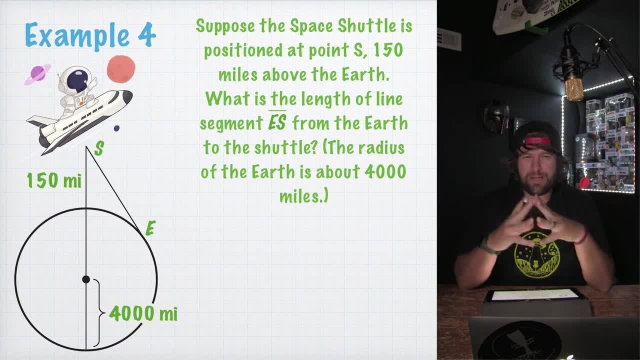 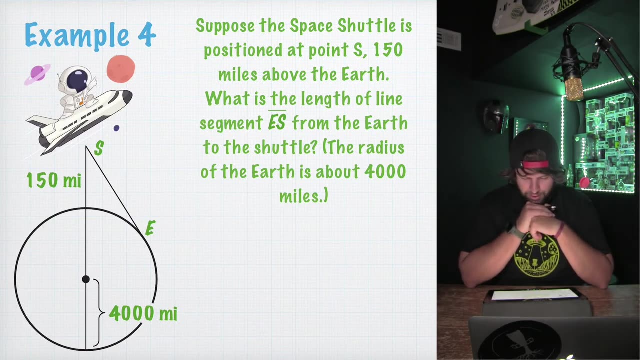 I'm starting to notice a trend with these space shuttle problems, and it's that they're a little longer than all the rest of the problems. So tighten your boots and realize we're looking at a space shuttle. Suppose the space shuttle is positioned at point S, 150 miles above the Earth. What is the length? 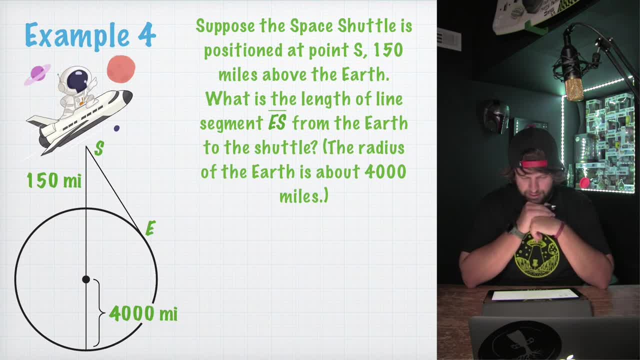 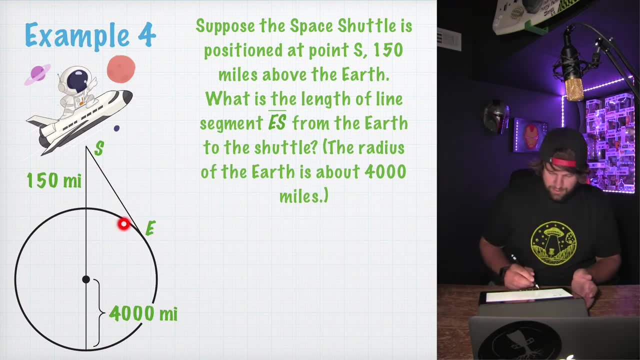 of line segment ES from the Earth to the shuttle, The radius of the Earth is about 4,000 miles, So we know that we're solving for SE and we know SE squared equals 150 times 4,000 plus 4,000, or. 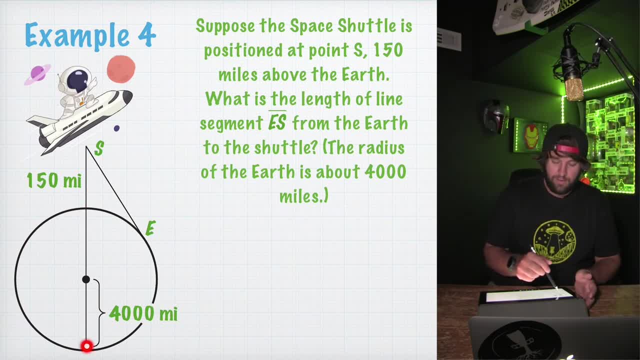 this would be 8,000 clear across the Earth, since the radius is only 4,000.. So let's go ahead and just write that down: X squared equals 150 times 150 plus 8,000.. Okay so X squared equals 150. 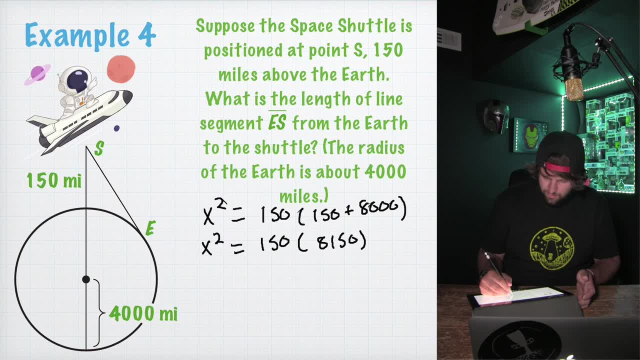 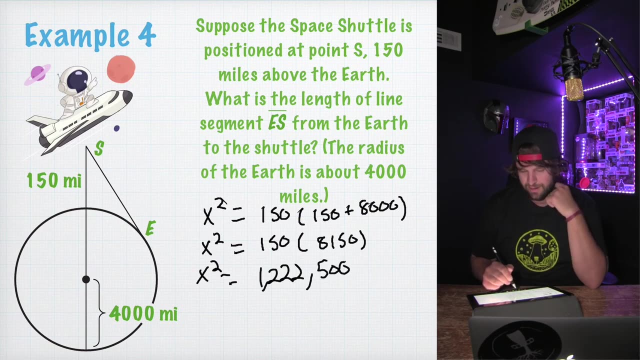 times 8,150.. 8,150 times 150 is 1,000,000.. X squared equals 1,222,500.. Okay, To finish solving this, we would take the square root of each side of this equation to cancel this out, And X is going to equal rough.